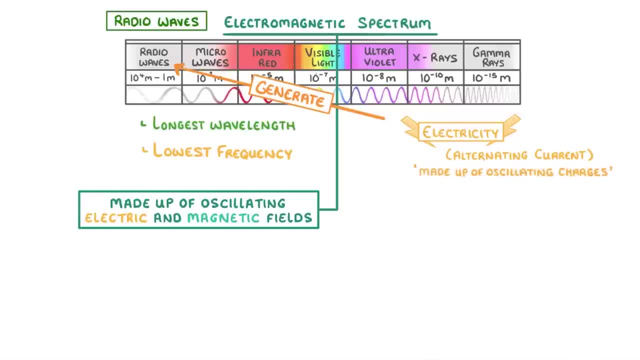 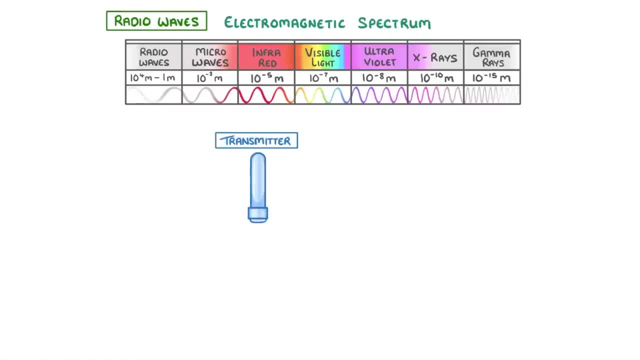 currents are made up of oscillating charges. To do this for very radio waves, we use a device called a transmitter, which is normally connected to an oscilloscope. The oscilloscope allows us to see the frequency of the alternating current that we're using. 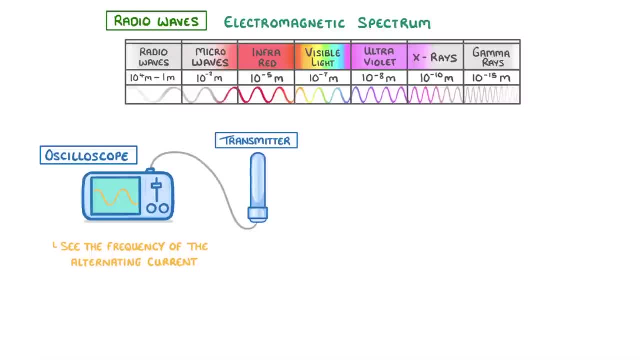 because we can see the frequency of the wave on the screen, And the reason we care so much about the frequency is that it's the frequency of the alternating current that determines the frequency of the wave that we're going to produce. Once the radio wave has been generated, we can detect it again by using a different device. 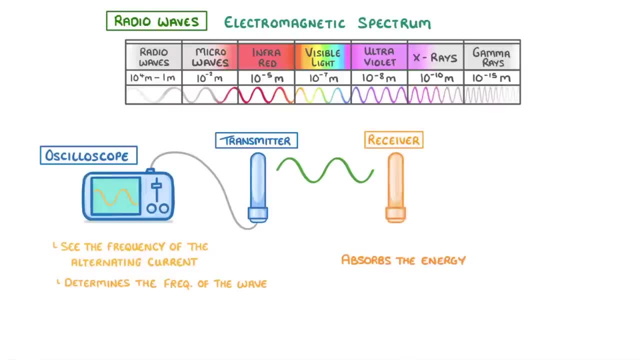 called a receiver, which absorbs the energy and generates another alternating current which it displays on another oscilloscope. The key point to understand here is that the frequency of this alternating current that it produces is the frequency of the wave that we're going to produce. 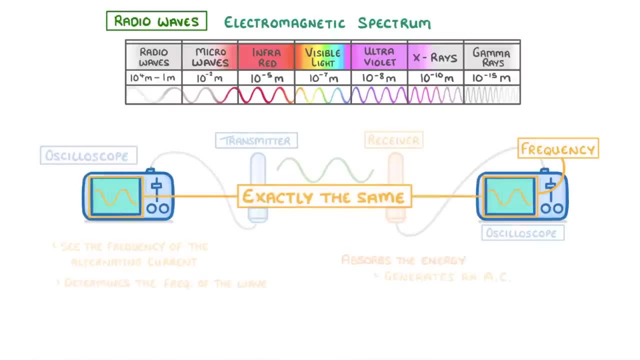 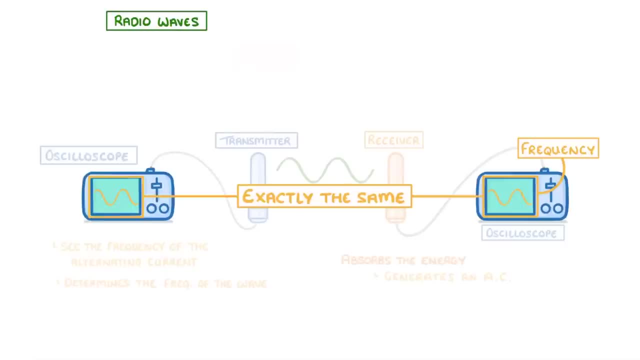 This is exactly the same as the frequency we used to generate the radio wave in the first place. This concept effectively allows us to transfer information because, for example, if we wanted to communicate the number 800, we would just generate a wave that has a frequency of 800. 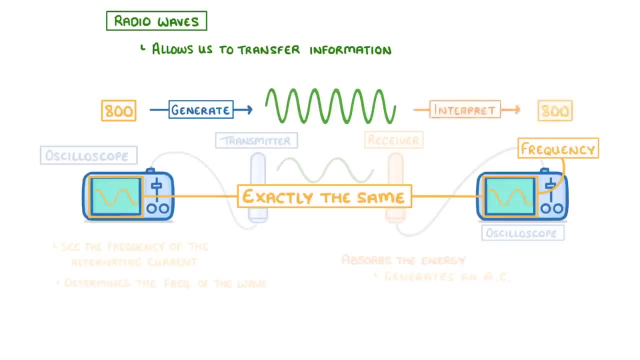 Hz, And then anybody with a receiver could interpret it. So we've effectively transferred the number 800, using alternating currents and radio waves, And the cool thing is that we can use this basic method to transfer information of pretty much any kind, not just basic numbers. 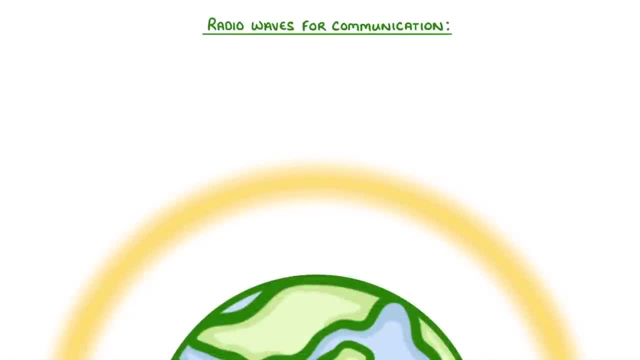 In fact, the main use of radio waves is for communication, and there are three types that you need to know about: Long wave, short wave and very short wave. Long wave radio waves can be transmitted huge distances, like from London to Singapore.